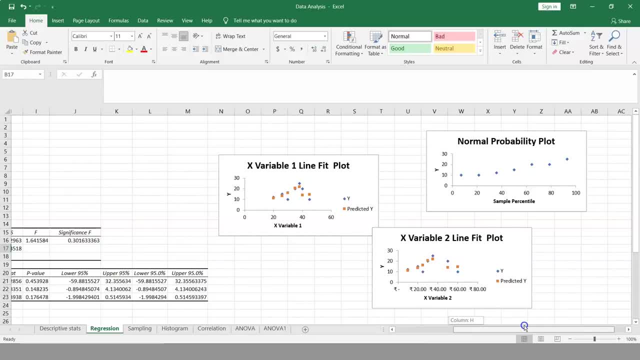 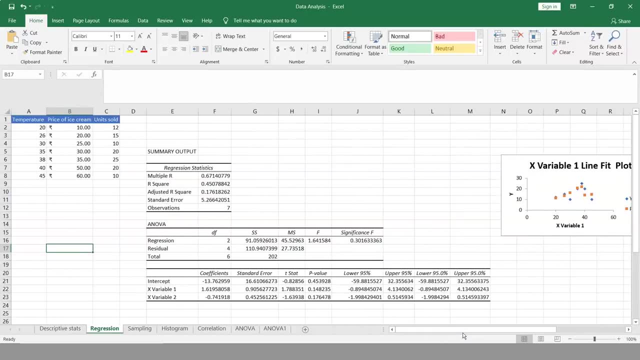 X, variable 2, and then you have normal probability plot. Now we have already seen how you can have your add-in, that is, data analysis, which helps you in doing different kind of data analysis here right Now. how do we do this? 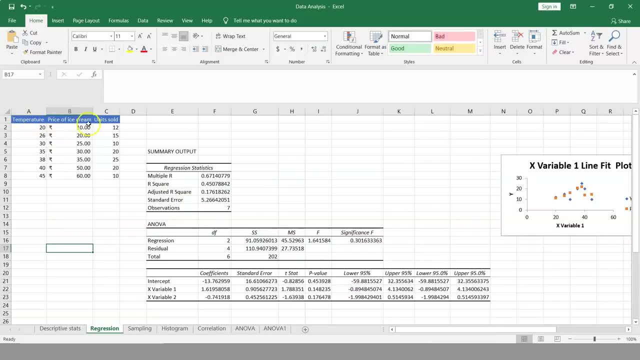 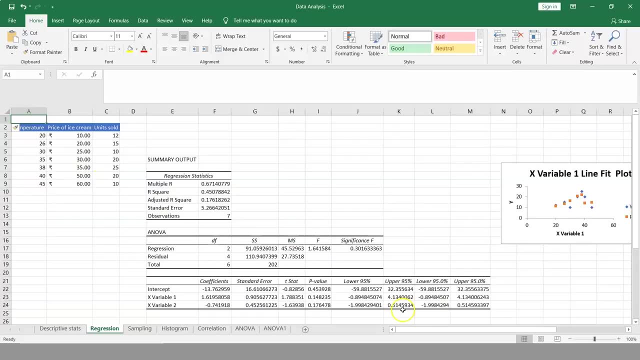 So we have our variables here, which is temperature, price of ice cream units sold, and when we talk about regression, we need to understand which one of these are independent variables, which one of these are dependent variables, right? So when you talk, 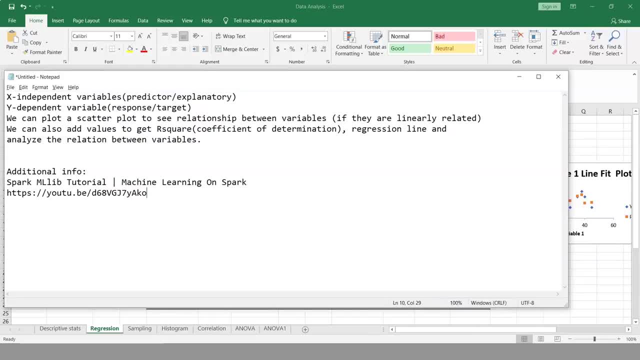 about your X. that's your independent variable, or we can say predictor or explanatory. So when you talk about your independent variables or, as we say, predictors or explanatory variables, these are the factors that might influence the dependent variable. And when you talk about 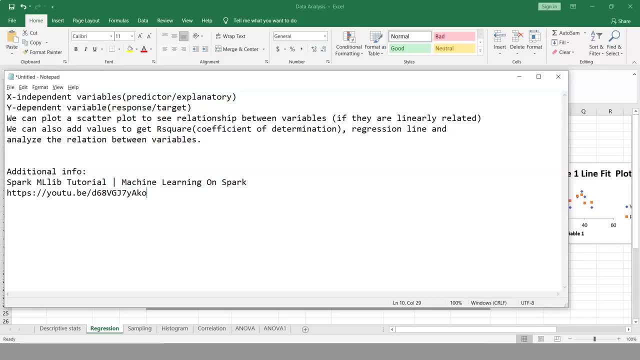 dependent variable. that's your response or target. that's the main factor you're trying to understand or predict. So we can plot a scatterplot to see relationship between variables if they are linearly related, are they positively related, negatively related, and so on. We can. 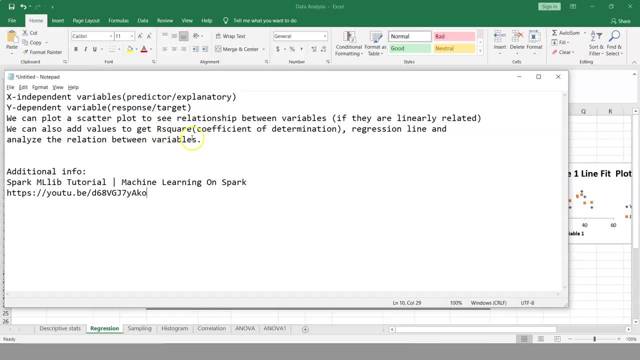 also get variables that are linearly related. are they positively related? negatively related values such as R-square, which is coefficient of determination, regression line, and then analyze the relationship between variables. So here is one of the links of one of my 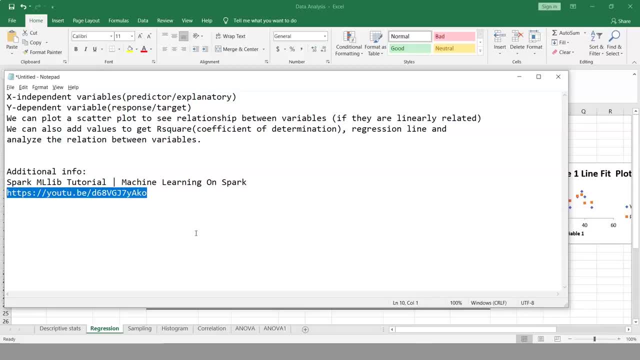 other videos where we are learning on machine learning and also on regression, but that's programmatically and using a processing framework such as Spark. Now here let's see how do we do this in Excel. So basically, we would want to use our variable. 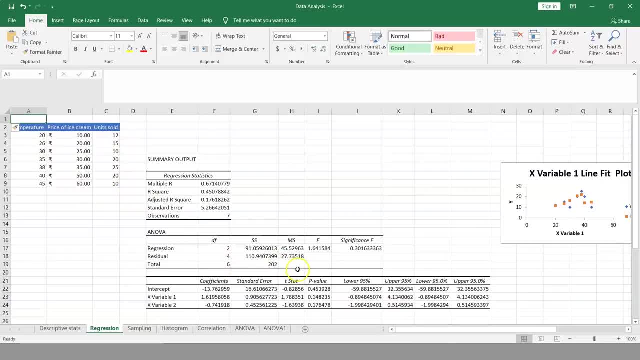 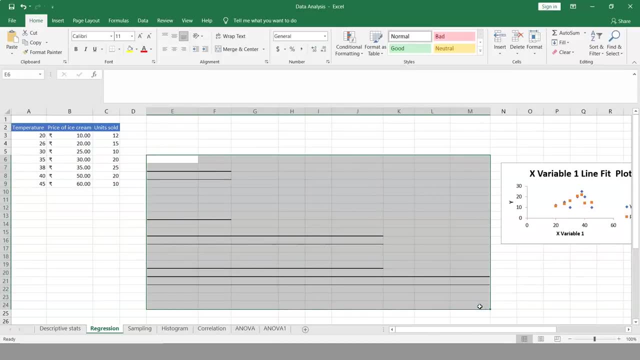 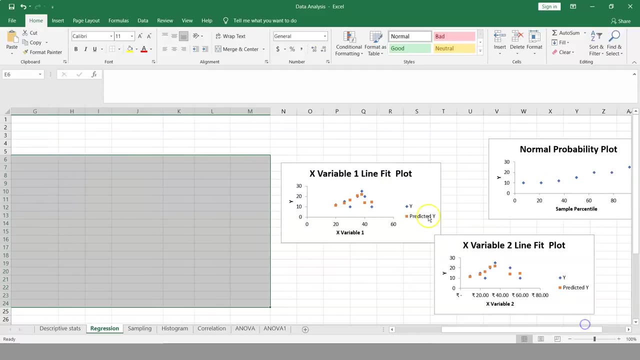 which is temperature price of ice cream units sold, and then get these plots. So what we can do is, for example, I can get rid of this and might be- I can just say no borders- and when it comes to these plots, we can have them generated again- That's not a big deal- using your data analysis. 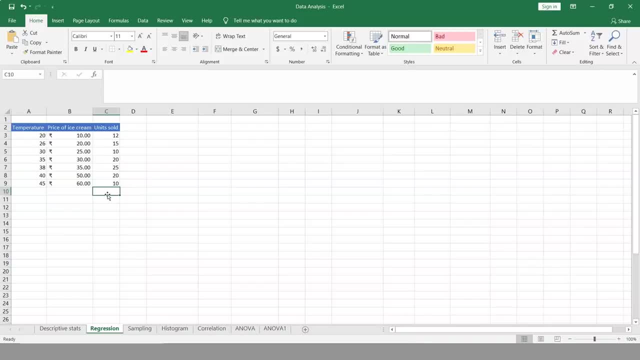 add-in tool, So we have been given variables here. Now, as I said, when we talk about your regression analysis, we need to understand whether we have one variable or we have multiple variables. right? So you might have heard of univariate analysis. 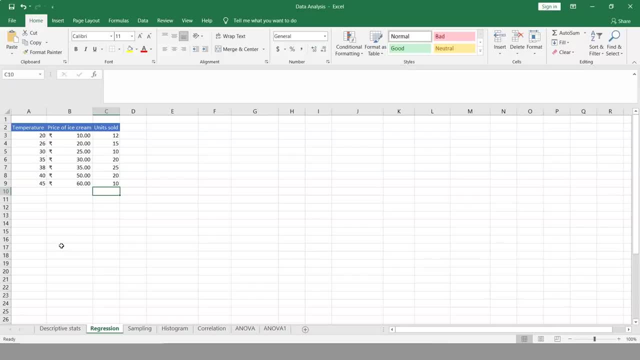 bivariate analysis and so on. Well, here we are focusing more on using Excel to do our regression analysis, So I'll not go deeper into regression topics, but certain things as basics should be known That when we talk about regression analysis, what does it do? It helps you understand how the 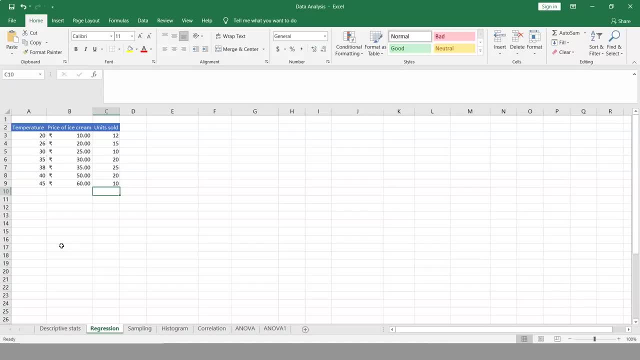 dependent variable changes when one or more independent variables vary And it basically allows us to mathematically determine which of those variables really has an impact. So, technically, when we talk about regression analysis model, that is based on the sum of squares and we can use that to determine the dispersion of data points. So basically a mathematical way to. 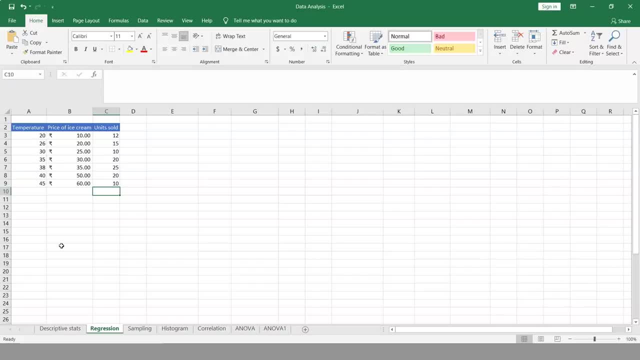 find the dispersion of data points. So mainly the goal of the model is to get the smallest possible sum of squares and draw a line that comes closest to the data. So that's what we mean by our regression line, or basically looking at the points and seeing if the points fall on a regression line. 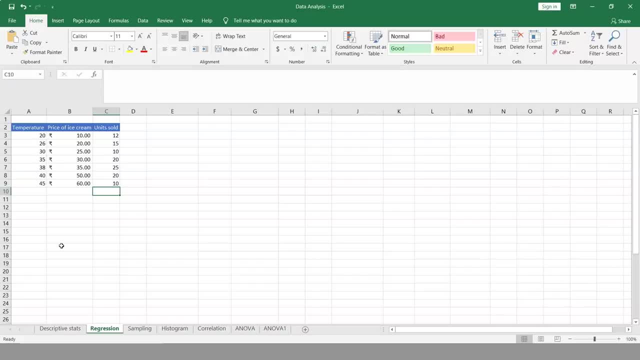 if there are residuals, that is, points which do not fall on the regression line, and we can measure the points line. And in terms of statistics, when we talk about statistics, we differentiate between a simple and multiple linear regression. So you have something called a simple linear regression. 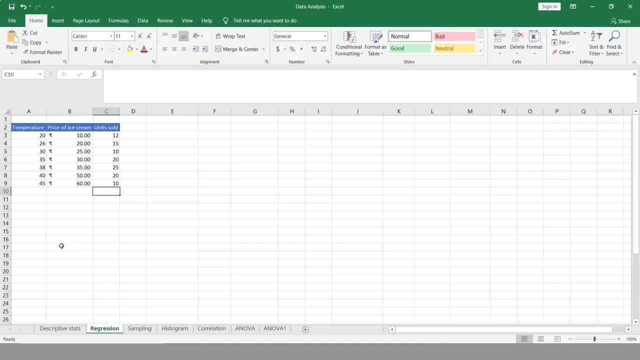 models, which basically gives you the relationship between dependent variable and one independent variable using a linear function. And if you use two or more variables, that is explanatory variables- to predict the dependent variable, we are actually dealing with multiple linear regression. So if the dependent variable is modeled as a non-linear function, because the 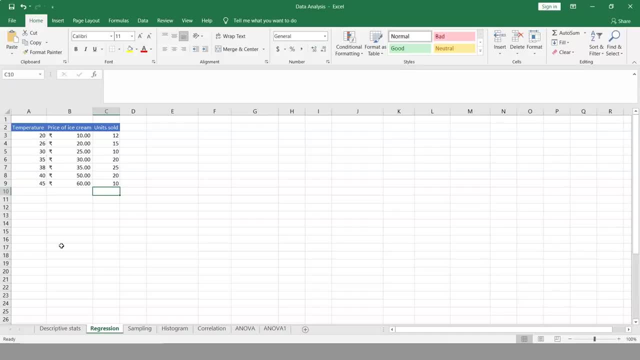 data relationships do not follow a straight line. we have to use non-linear regression. Now, what we will do is: we'll see how we can work on this. So here we have some variables And if we look at this, it might be based on temperature. price of ice cream. 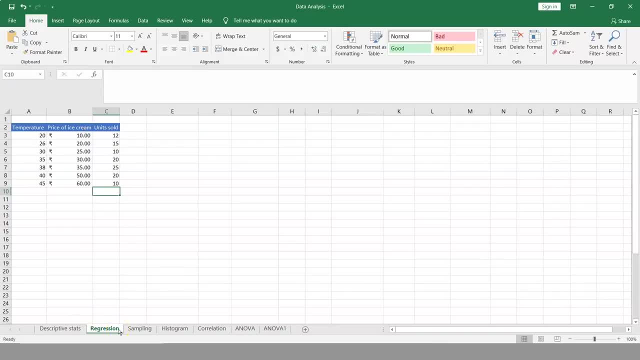 we would want to find out how many units were sold. Now what we can do is we can basically start looking in by creating a simple scatter plot, which is quite easy in Excel. So if you have been given variables, what you can do is you can click on insert. You can then choose the kind. 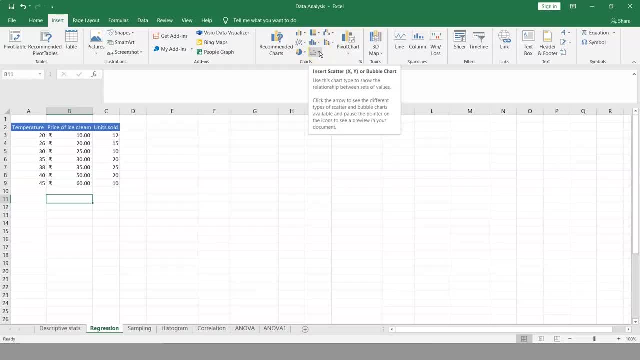 of plots which you want, And here you have insert scatter plot, So we can choose this, And you can choose the first option. So that gives you a blank layout, And what you can do is now you need to select data. So, for example, let's click on select data. 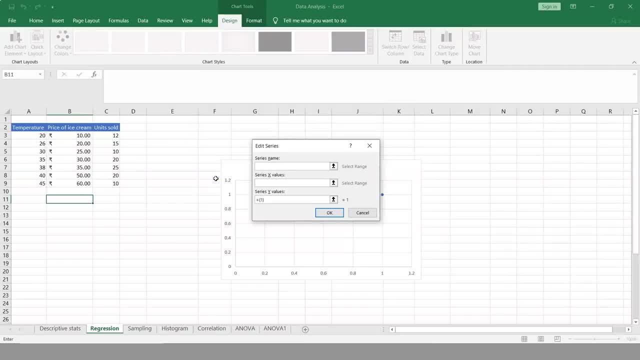 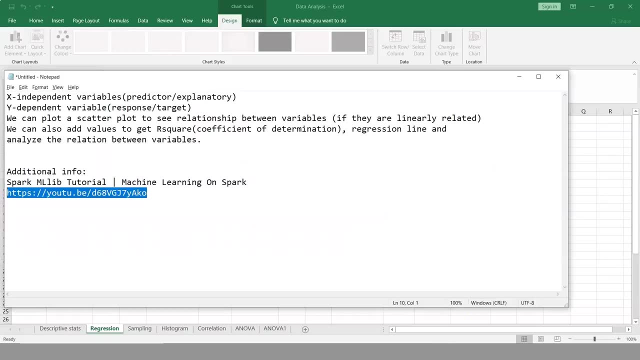 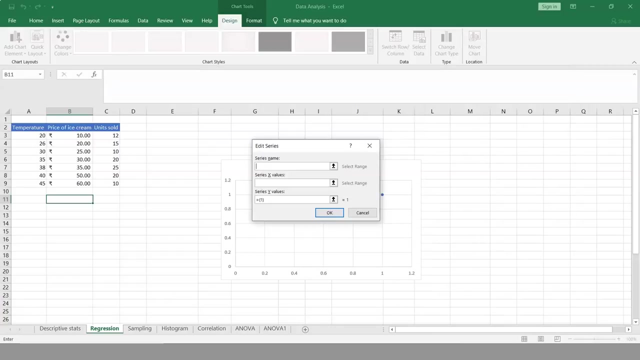 And then you can say add. So what we would want is we can give a name. So we want x values and we want our y values, right? So when you talk about y, that's your dependent variable or your response or target. So that is in our case, units sold And x values are one set of features or variables. 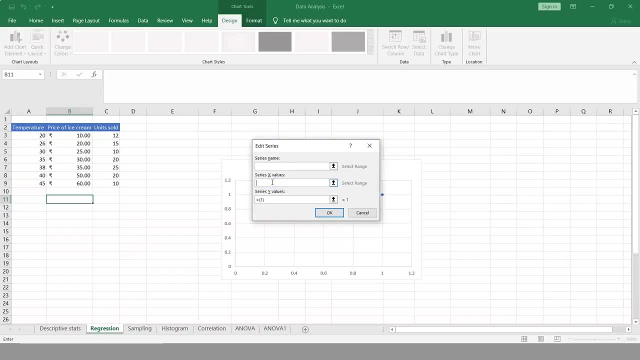 or variables, So we can give a name, So we can give a name. So we can give a name, So we can give a multiple variable. So here I can click on this series x values and then I can select this Now in y values. what I can do is I can select these and then I can just say OK. So that shows. 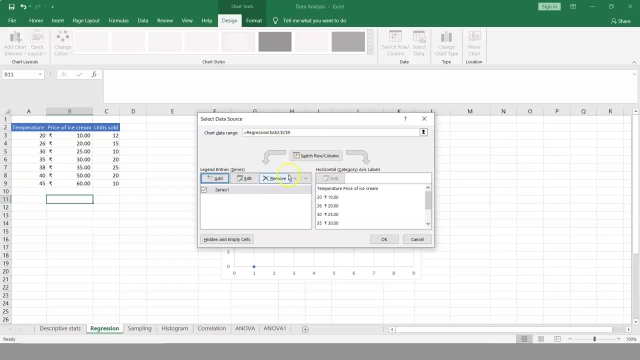 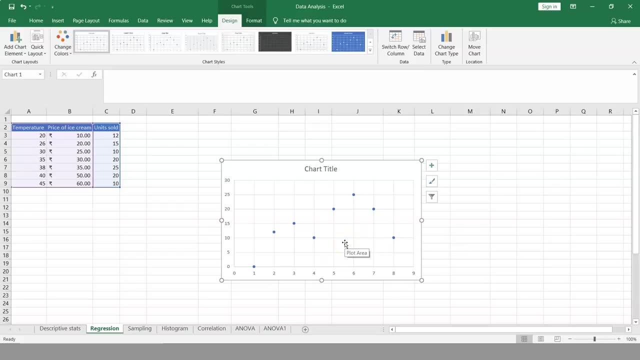 me that it would be giving me a regression scatter plot. Now let's say OK, And we have some points plotted here. Now, if you would want to see the impact of one individual scatter plot, you can do that. If you want to see the impact of one individual variable, such as temperature or price, 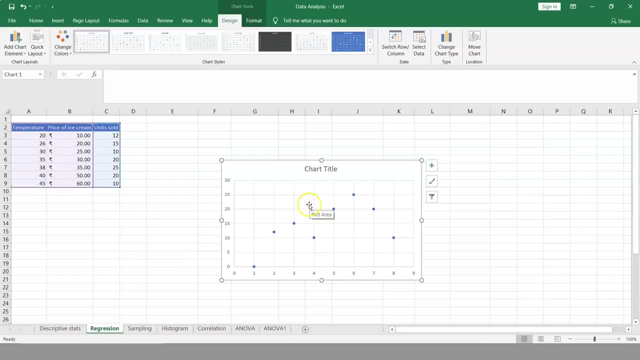 of ice cream. you could as well do that. Now, what you can also do is you can add more meaning to this by giving in a title, or you can also go into quick layout and you have various options here. So you see, it gives you what is the axis title, what is the series, And I would prefer to use 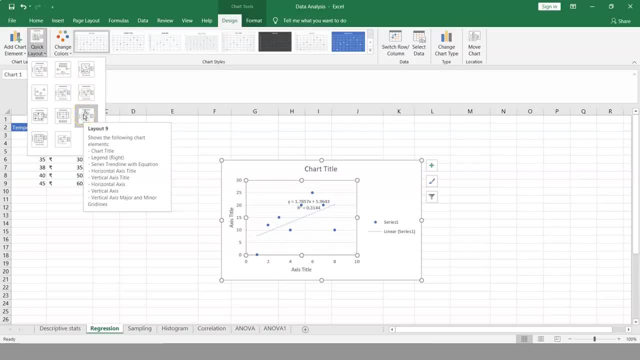 here something like this one. So that gives you your regression line, That also gives you your R square And that gives you your y and x. That is your coefficients. So let's select this one And then we have some values which we can use to compare. This also shows me the regression. 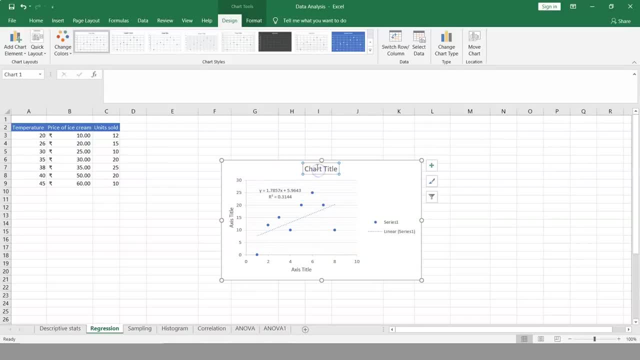 line And you can keep this for reference. If you would want, you can change the chart title to something else, say scatter, plot of dependent, where it's independent Variables, and you can give any name which has more meaning and we can get rid of this one. So we 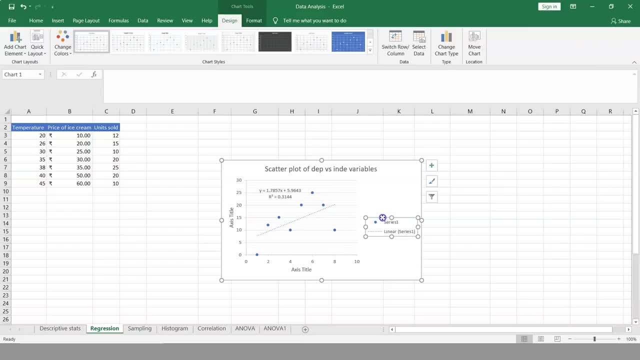 have series and we can say: what are these points, if you would want to add in legend, If you would want to do that, or I can just get rid of this and I will keep these values here, which will see when we do a data analysis. We can always compare these values. So here I've created 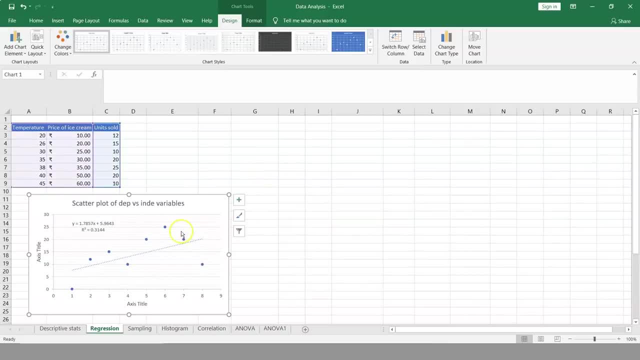 So here I've created a simple scatter plot and then I can look at dependent vs independent variables, or I could have selected one particular variable. so this is just for reference. now we can add more details. we can say: what is my x axis, what is my y axis? so basically you can here say, for example: just say y. 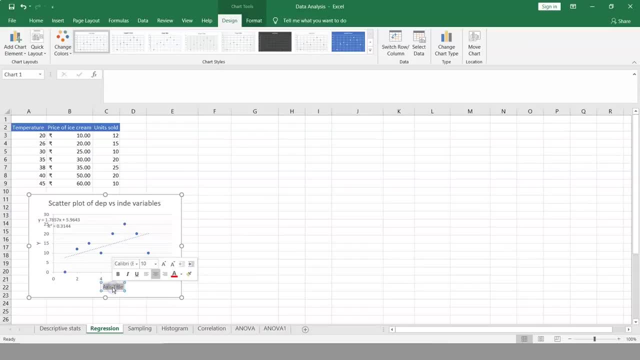 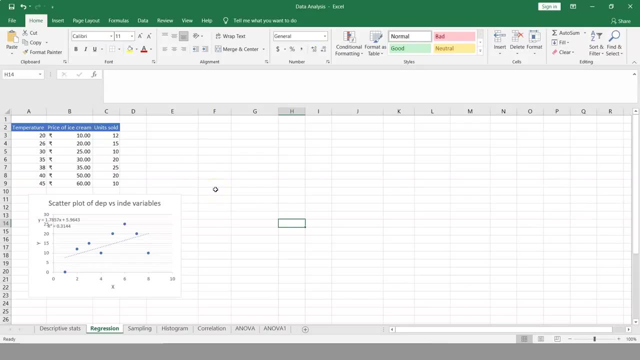 and might be here. I will say x and we can rename that later now. how do we perform data analysis or get into regression? right now, what we would want to do is we would want to get or we would want to do the regression analysis to demonstrate the relationship between dependent and independent. 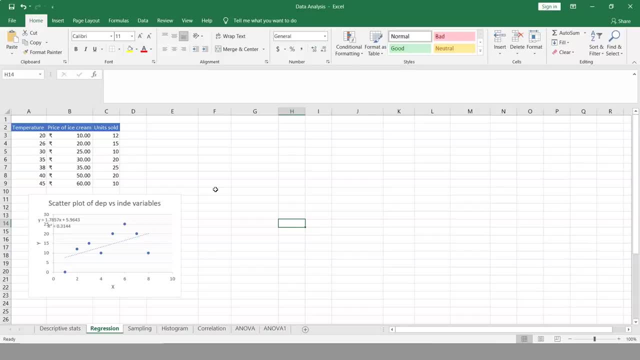 variables. so normally when you talk about your linear regression equation, you might have known about it. so it is basically y. when you say y equals, you can say bx plus a plus c, and this would be normally the mathematical equation for a linear regression. where x is your independent variable, y is your dependent variable. 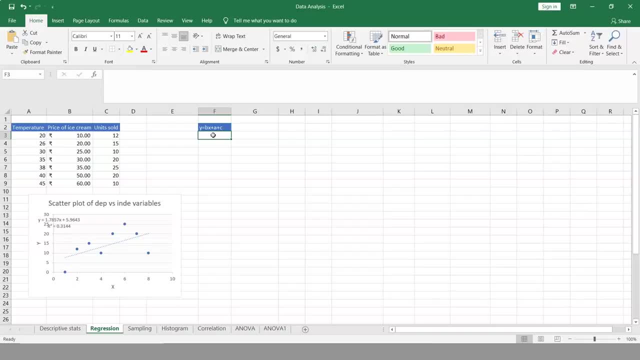 your and I have your constant right. so that's your sorry. that's basically your random error term, right, which is basically the difference between the actual value of dependent variable and its predicted value. so your linear equation always has an error term, because in real life predictors are: 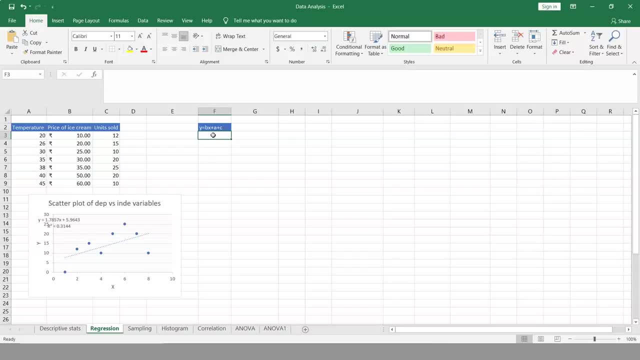 obviously never perfectly precise right now. what we can do is we can also reduce this equation to: y is bx plus a, and that's the equation of a line. we can look into this and the linear equation can be understood mathematically in this way. now, how do we do it in excel? so what we can: 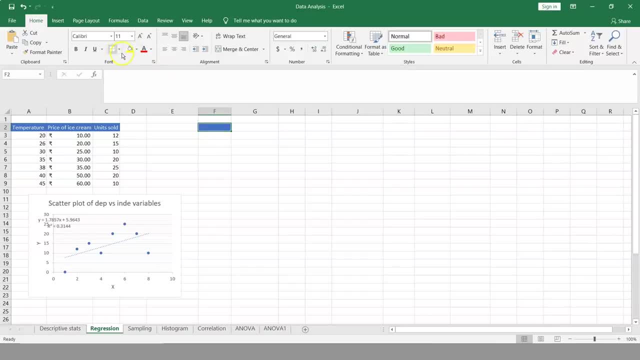 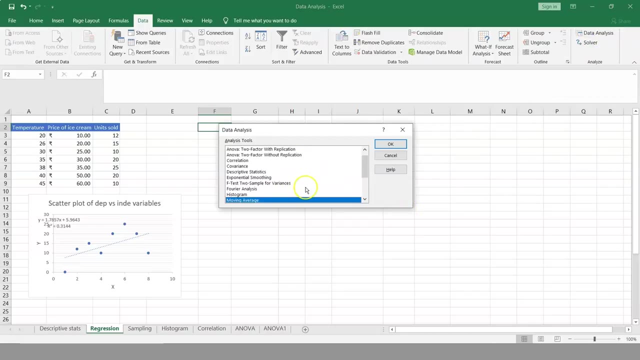 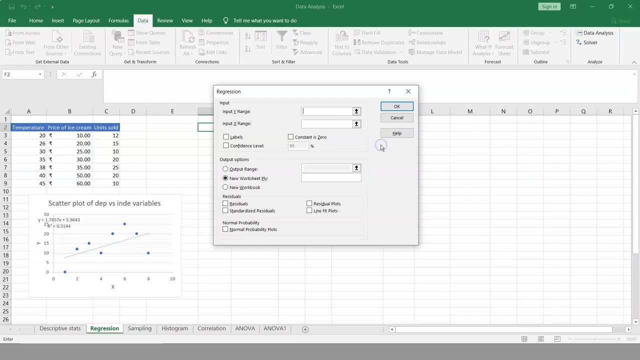 simply do is here, let me. yeah, so we need to get into data. and then here we have our data analysis add-in. you can click on this one and from these different options you can choose regression. so that's what we would want to do. now we'll say: okay, now here you need to give your input y range, so as 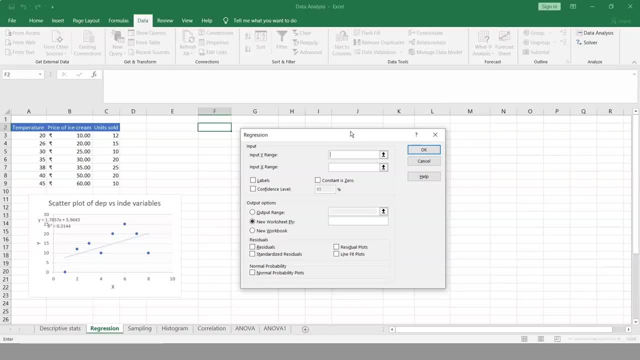 I said, you will have to select the dependent and independent variables, right? so we would want to do some regression analysis here and here we have your x and y, so, y being your target value, that's basically your units sold. so we can select this, along with the labels when it comes to x. 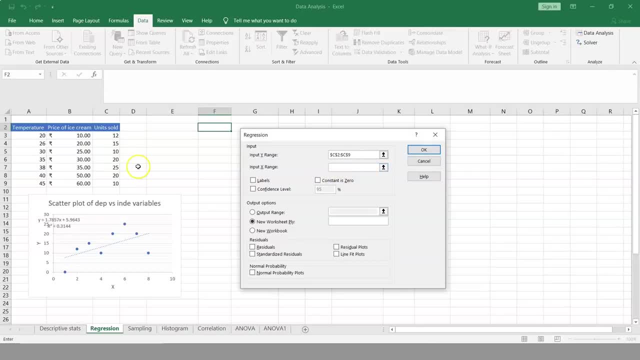 either you can select one variable or multiple variables. so I will select temperature, price of ice cream and then, since we have chosen the headings, we will go for labels. right now we can always look at the confidence level. we can change that, so you can say whether you want it in a new. 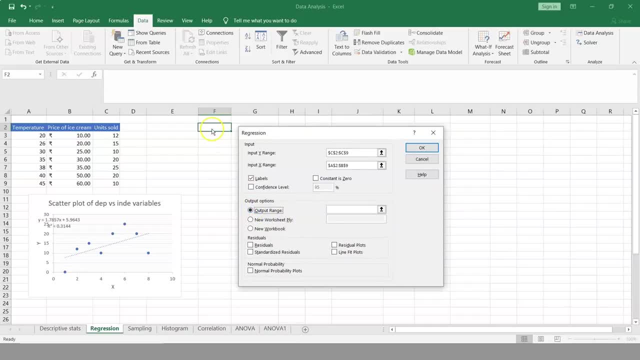 worksheet, or you can just say how much you want it to be, and then you can just say how much you want it to be and you can select your output range, and I will probably just click here and select one of the cell here. now we can also choose the other options which we would want to see as a part. 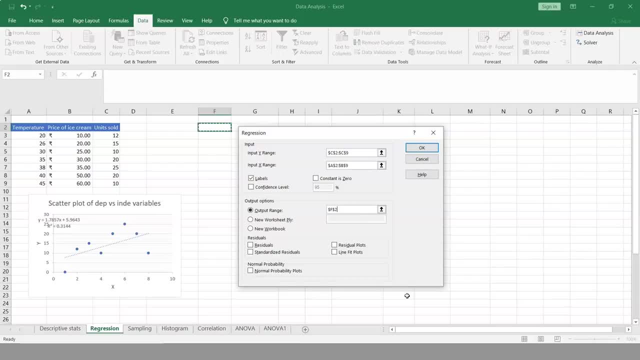 of this regression analysis. so, basically, we have selected input, y range, which is your dependent variable, you have selected X range, which is your independent variable, and if we are building a multi regression model, then we have chosen temperature and price of ice cream, both. now we can choose the labels, which we have done. 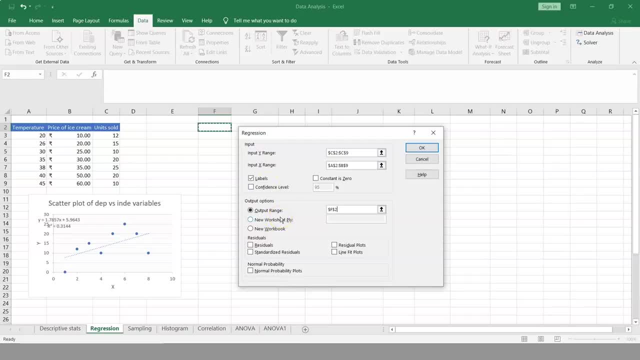 we can choose your output range, which is basically on this sheet, and then we can select the residuals, so that basically gives you your residuals. now we can also get your line fit plots, which you were seeing earlier. you can also go for your normal probability plots and then basically just 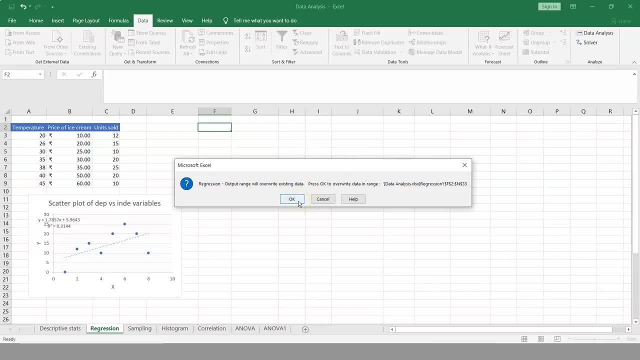 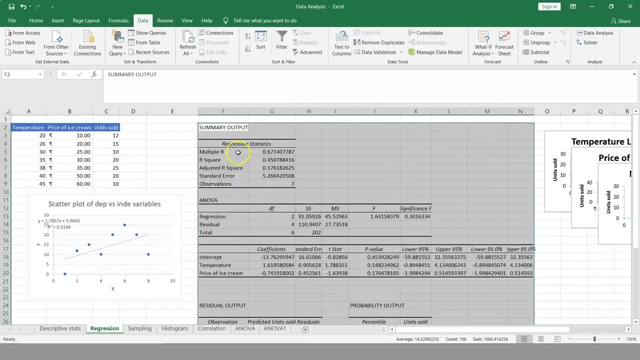 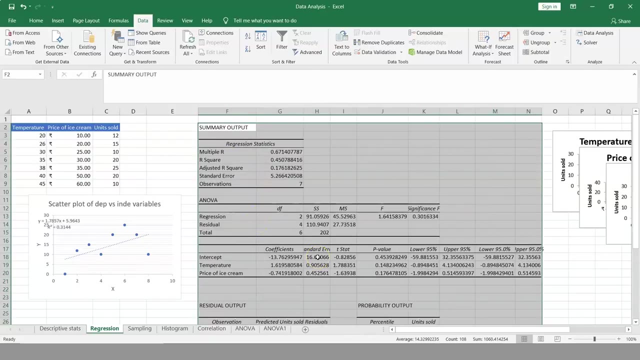 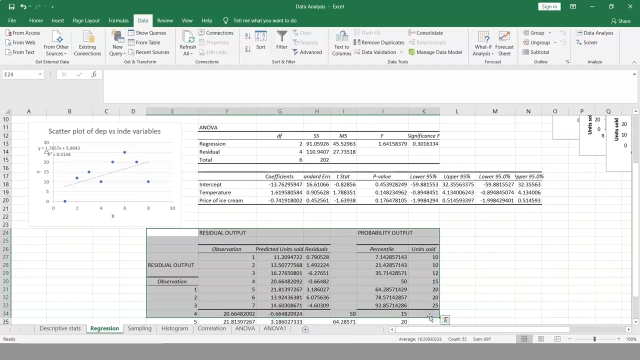 say okay and let's say okay and that basically gives you your regression analysis output. so we basically have your summary output. we also have anova. we have our residual output, that's from the previous one and basically we can get rid of this. that's not required. i can get rid of this one. 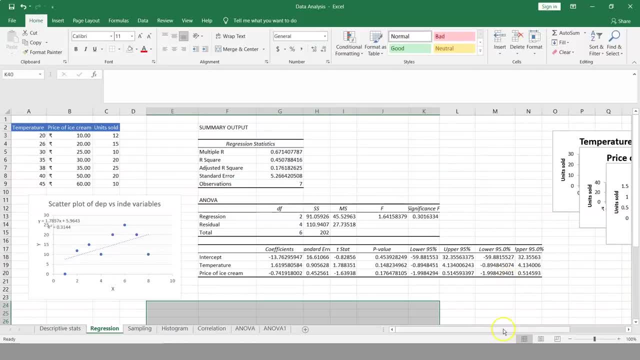 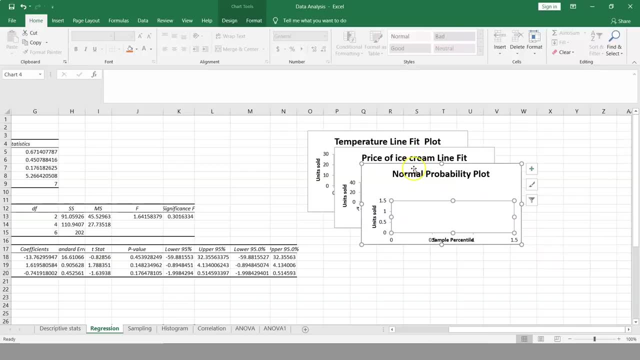 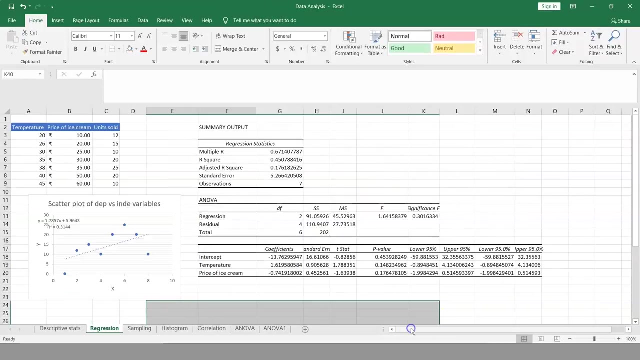 yep, so now we have our regression statistics. we also have our plots, so we can basically look into these. so we have our normal. let's get rid of these, let's get rid of this, let's get rid of this, and then what we can do is, since we had some existing data, it has overwritten. so let me get rid of this and 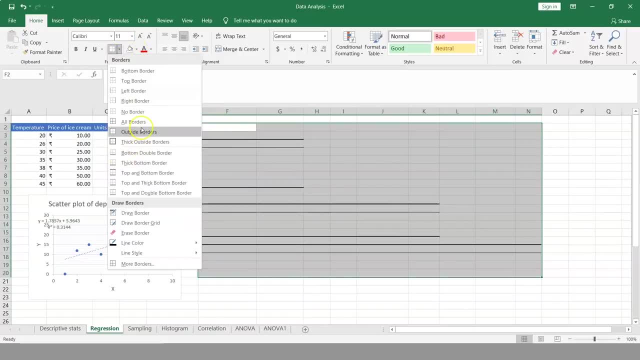 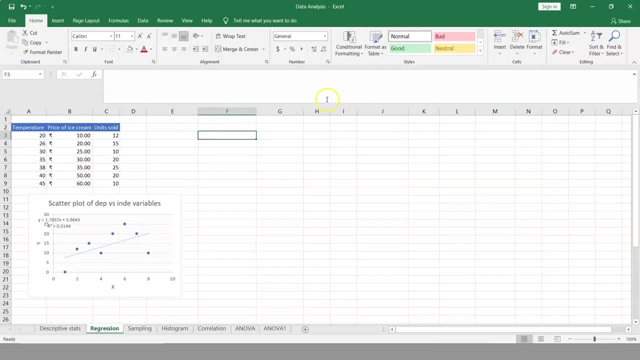 i'm going to go ahead and select the regression statistics and then we can choose our normal. I'll repeat this step again and let's say: no water, yeah. so now what we want to do is we want to do regression analysis. so we go get into data, we get into data analysis, we choose regression. 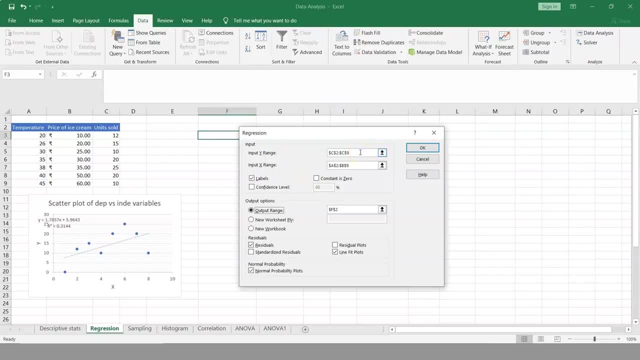 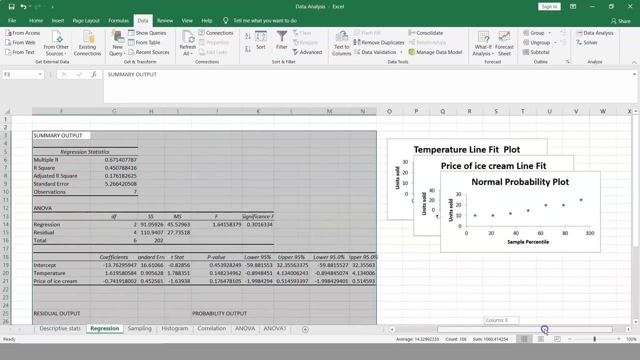 we have already chosen our y range, which is column c. x range is multiple variables. we have gone for labels output range, which we would want to select a particular cell. so let me select this. i'm going for residuals, line fit plots, normal probability plots, and say okay, so now we have 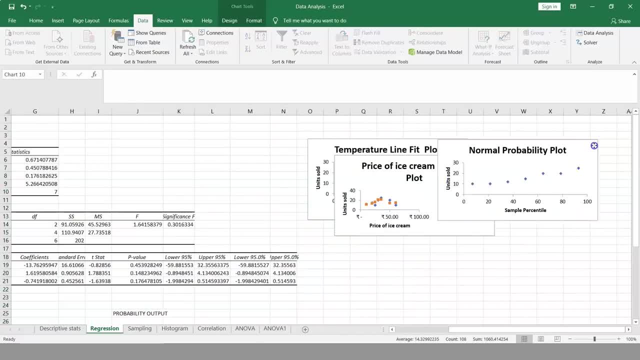 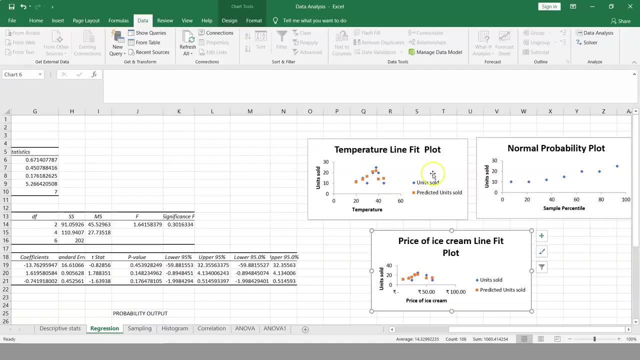 our plots. we can just separate them to have a better understanding. yeah, and that basically shows you the variables. so here it shows me units sold, and then what are the predicted units sold? and here the variable is temperature. here the variable is price of ice cream. right, so that's your one variable and second variable, and then you also have your normal. 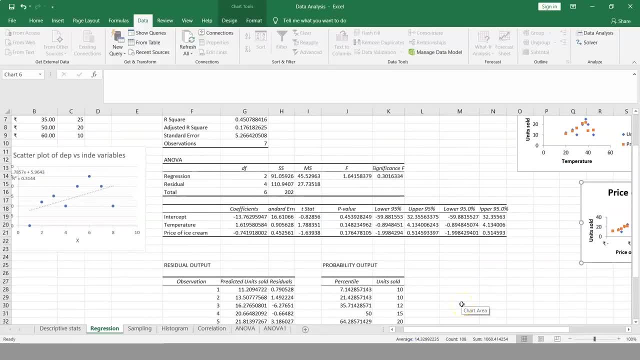 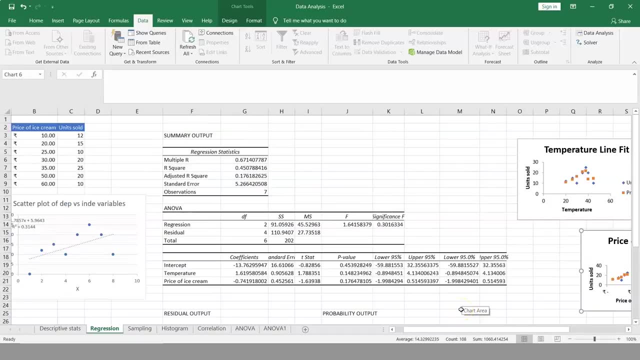 probability plot. now to interpret this, or to understand what we have here, where we look at your summary output. so it is good to understand what excel is helping us out. so, basically, when we do a regression in excel, it is performing all the calculations automatically. the interpretation is something: 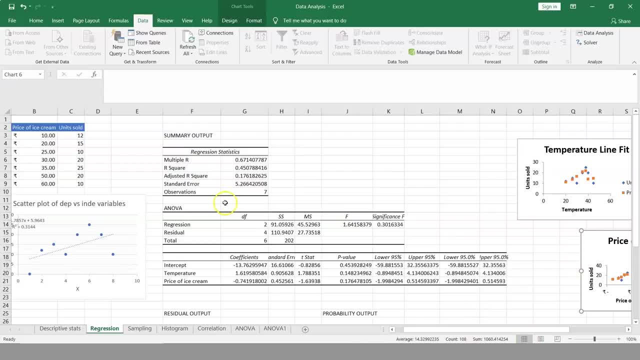 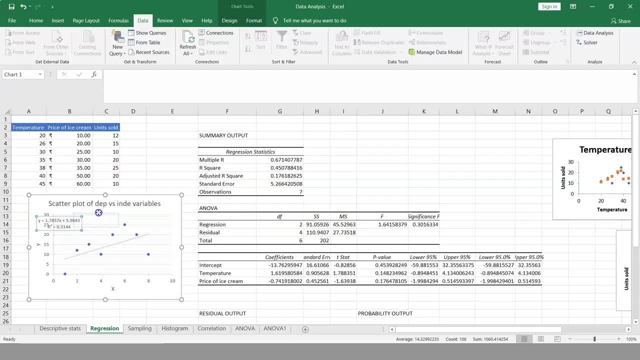 which we need to understand. so, basically, we are looking at multiple r value here and we can let's also fine tune this one. yeah, we have our values here and if you see, we have our r square now, we can then basically look at our multiple r. so what is your multiple r? that's your. 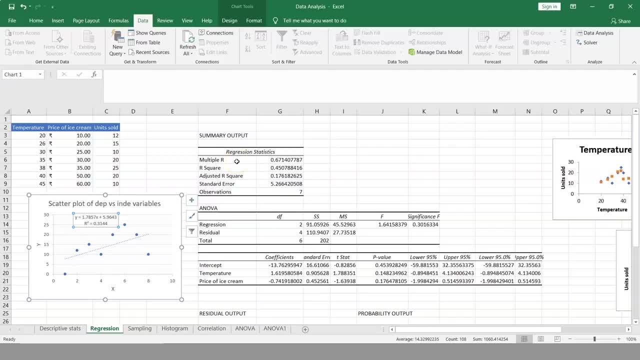 correlation coefficient, which basically measures the strength of linear relationship between two variables. so this can be any value between your. when you talk about your correlation coefficient, it can be any value between minus 1 and 1 and its absolute value indicates the relationship strength. so the larger the absolute value, the stronger the relationship. so one basically means a. 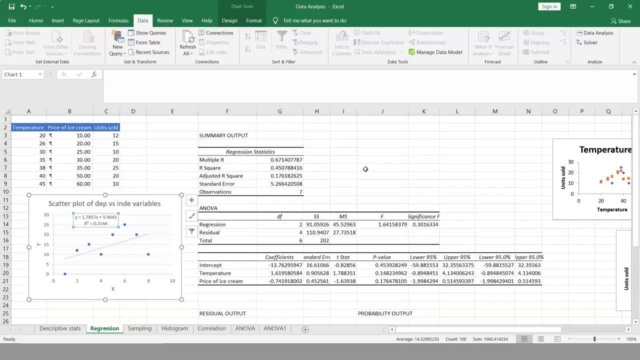 strong positive relationship. minus one means a strong negative relationship and zero means no relationship at all. now, when you are looking at r squared, that is the coefficient of determination, which is used as an indicator of the goodness of the fit. so it basically shows how many points fall on the regression line. 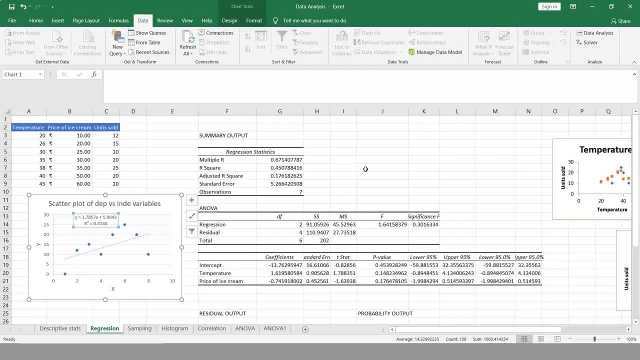 So your R square value is basically calculated from the total sum of squares. when we say precisely, It is the sum of squared deviations of the original data from the mean Now when we talk about looking at the value of your R square. so it is basically, we can be. 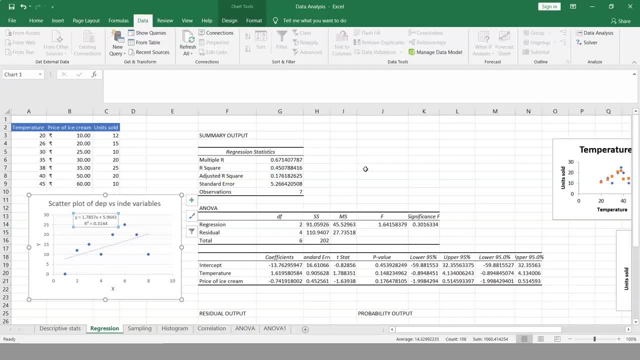 seeing that this is 0.450788.. That's the value which I'm talking about. So it basically means 45% of our values fit the regression analysis model. So in other words, 45% of dependent variables, that is, your Y values, are explained by the independent variables, that is your X values. 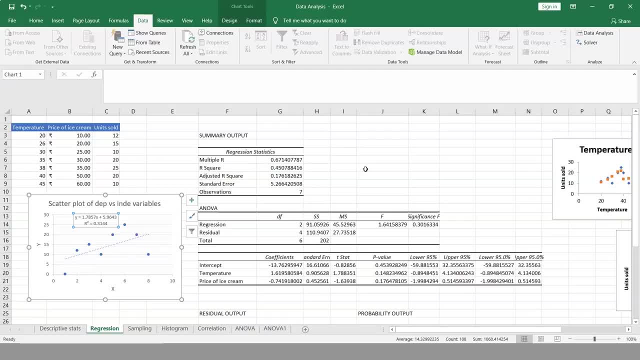 So normally if you have R squared values, if you have a value higher, then that is considered as a good fit, And here we have considered multiple variables. Now, when you talk about your adjusted R square, it is the R square. 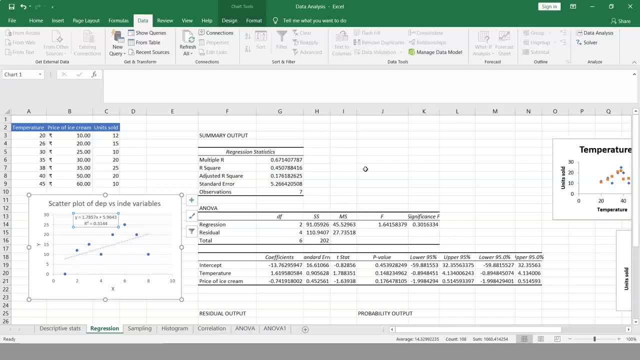 adjusted for the number of independent variables in the model. So you would want to use this value instead of R square for multiple regression analysis, such as in our case. Now you also have standard error, So that's basically goodness of fit measure that basically shows the precision of your regression analysis. So 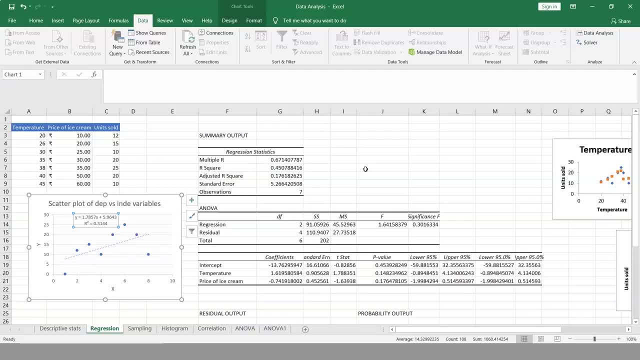 the smaller the value, the more certain you can be about your regression equation. So when we talk about your R square, that represents the percentage of dependent variables, variance that is explained by the model And standard error is basically an absolute measure that shows the average. 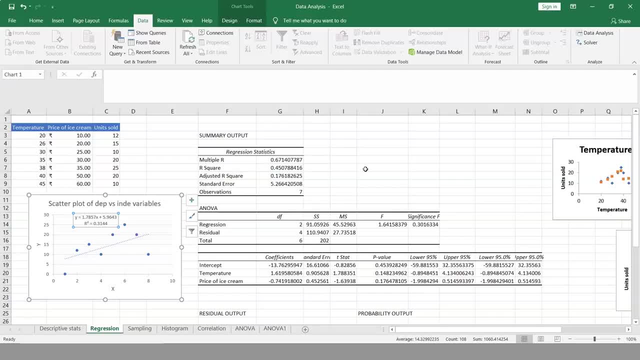 distance that the data points fall from the model. So that's basically the percentage of dependent variables from the regression line. So you will have to look back into regression statistics terminologies to basically understand more of this And, if you're already from data science. 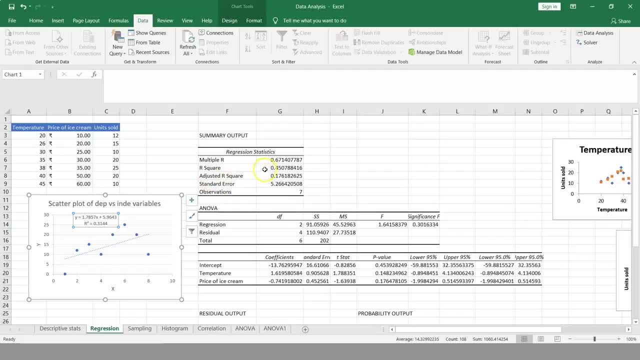 background, then you already know what I'm talking about. We are just seeing how Excel easily helps us in doing these things. Now we can also look at observations here, which is basically the number of observations in our model, which is seven. Now, when we talk, 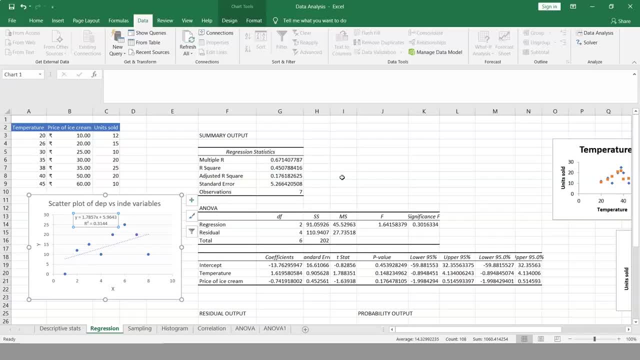 about regression analysis and if we look at analysis of variance, that is your ANOVA values here. So we basically see DF. you have SS, MS F and significance F Now to understand these. so basically what we are doing is, or what Excel is doing- is it splits. 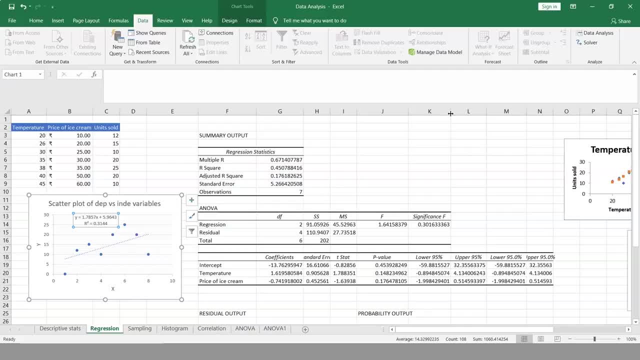 the sum of squares into individual components that give information about the levels of variability Within your regression model. So when you talk about your DF- that's basically the number of degrees of freedom associated with the source of variance- You have sum of squares. 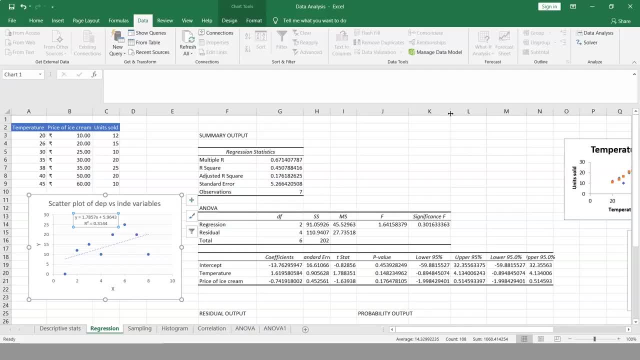 that is your SS. So smaller the residual SS compared with the total SS, the better your model fits the data right Now, when you talk about MS, that's your mean square. You have F is basically the F statistic, or you can say F. 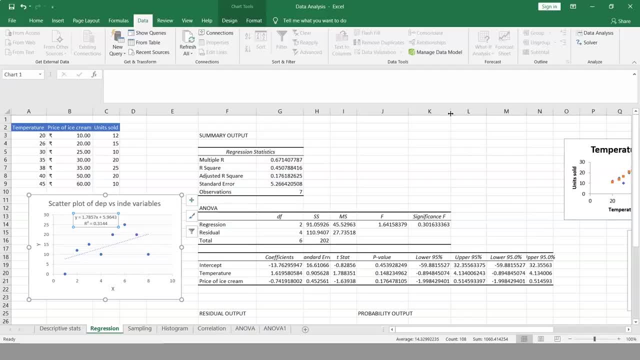 Test for the null hypothesis. Basically, it is used to test the overall significance of the model, And then you finally have your significance, F, which is the p-value of F. So when we usually talk about simple linear regression, the ANOVA part is not really used. 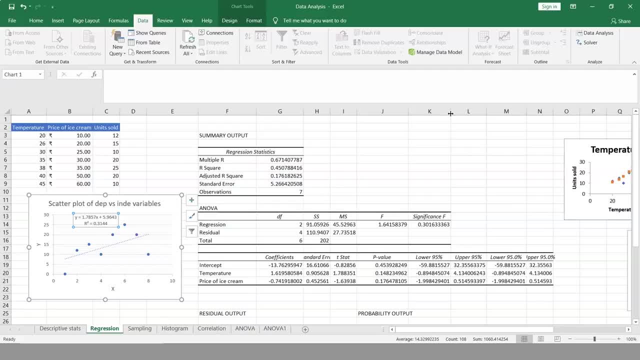 or it's rarely used, right? But when we look at the significance F, you can see that it's the P-value of F. So when we look at the simple linear regression, the ANOVA part is not really used or it's rarely used, right? But when we look at the significance F, it's. 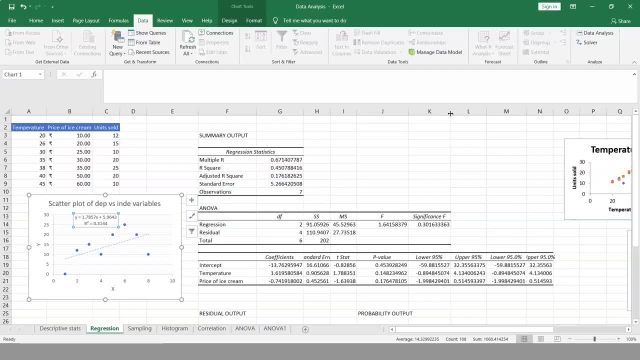 the P-value of F. That gives an idea of how reliably or statistically significant our results are. So if significance F is less than 0.05, that's 5%. our model is okay. If it is greater than 0.05, we will have to better choose another independent variables, right. 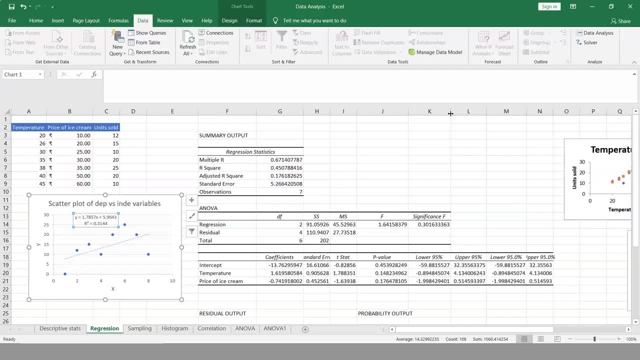 Now we can also look at the output of coefficient F. So we can also look at the output of coefficient F And that's what we would want to look at. So you basically have your intercept here. So when you talk about your intercept- temperature, price of ice cream- we know we are looking. 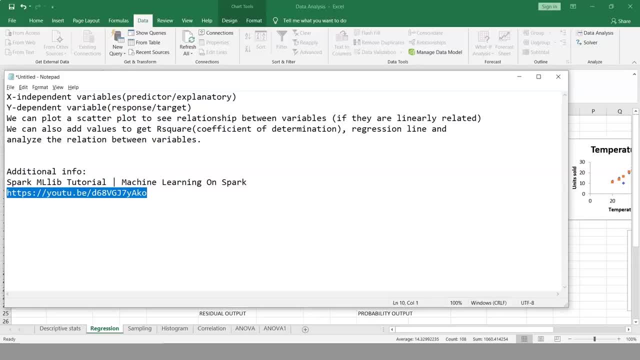 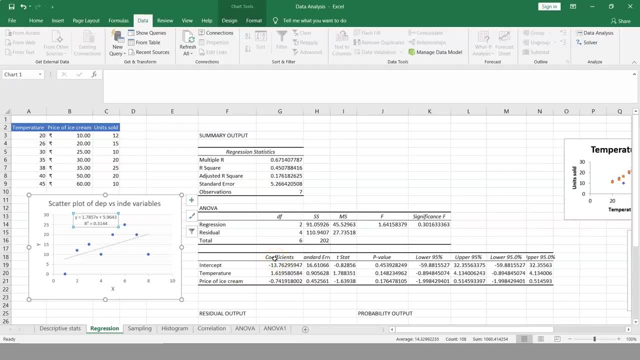 at our variables. So we know we are looking at our variables and then we are also looking at our intercept, which basically gives you more details on your coefficients. The main important thing when we talk about regression analysis is basically your coefficients. It basically enables you to build a linear regression equation in the form of y equals bx plus a, which 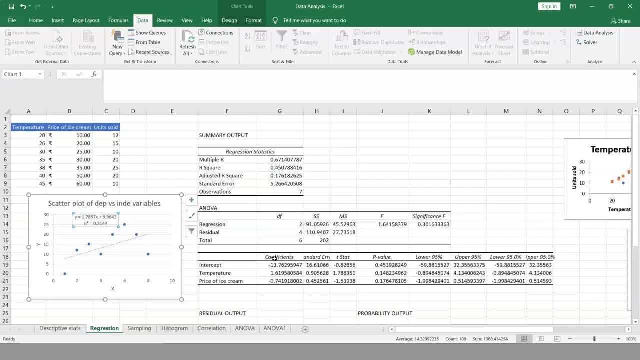 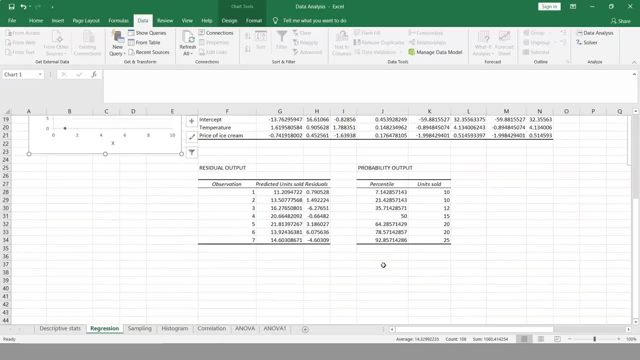 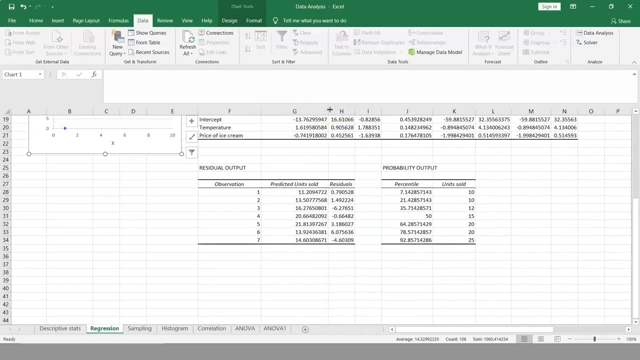 i explained earlier and then basically we can understand our regression analysis output better now when we look at the residual output which we are seeing here. so that gives you your observations, how many observations we have. it shows what is the predicted unit sold and then it also gives you your residuals so we can compare the estimated and actual number of sold umbrellas. 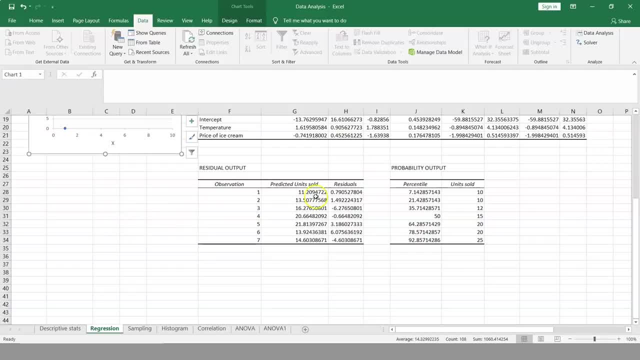 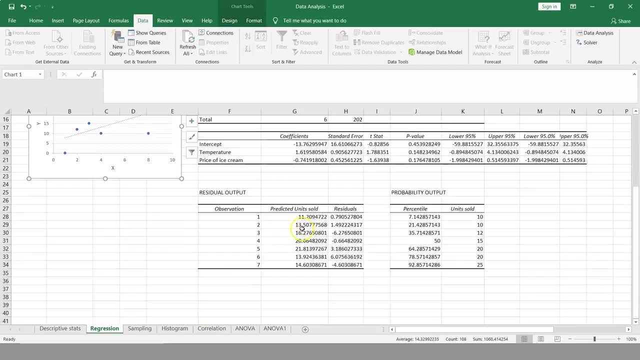 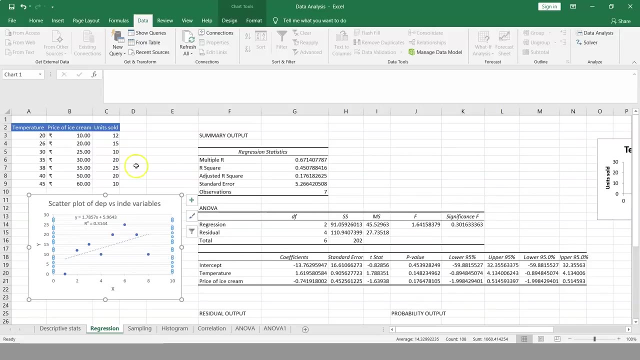 based on the observation. so we have 11.209 here and if you compare that's basically 12. the second one is 15 and here it is 13.5. you have, and similarly you can compare, all the values of actual units sold and what our regression has predicted. 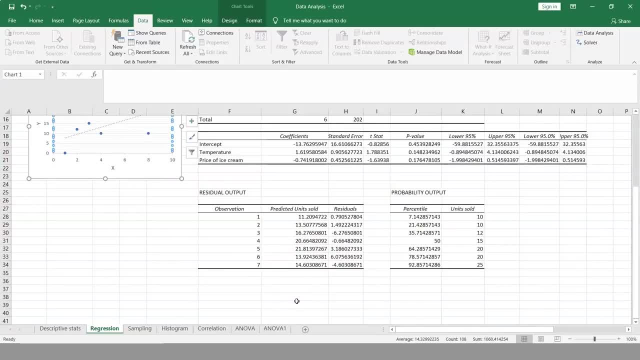 so basically what we can do is we can compare these and we will see if there is any difference or no. right, so obviously there will be or there would be some difference, because independent variables are never perfect predictors of your dependent variables and the residuals basically help us in understanding how far the actual values are from the predicted values. 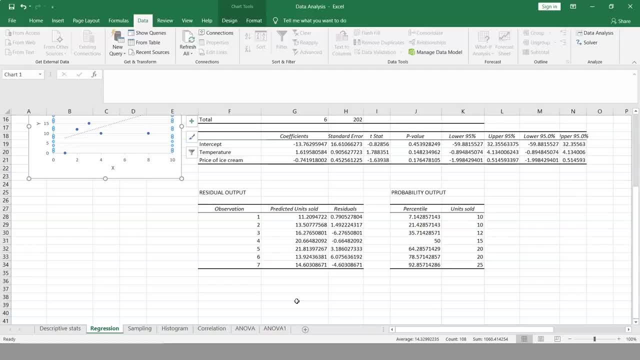 so that's what we see here in the residual section. so, for example, when we look at this one, which is 11.209 and the actual is 12, we see what is the residual and how far is the predicted value from the actual value. so similarly we can also look at the percentile values. so 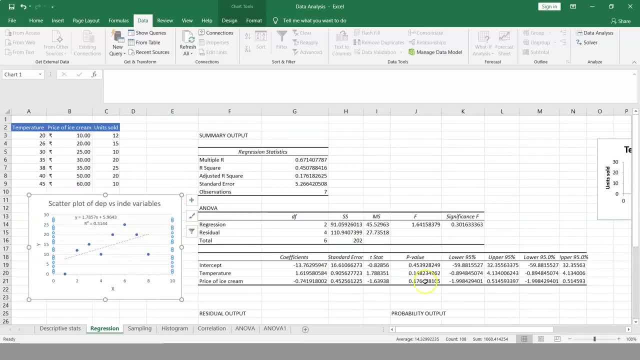 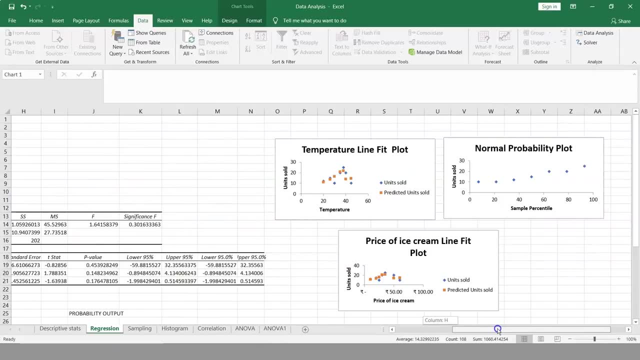 that gives you your probability output and this is what we have in our graphs. so we have basically our variables, we are looking at our variables and we are looking at our variables and also the units sold and the relationship between them. we can basically, uh, add in more. 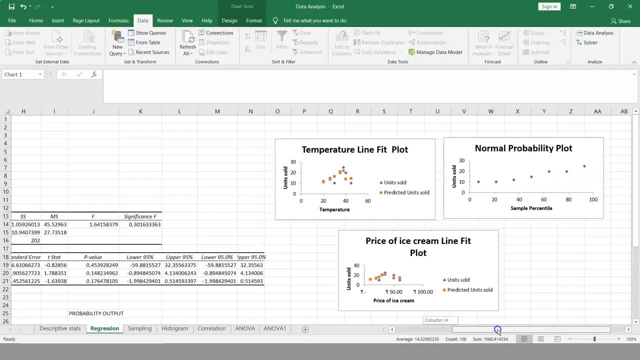 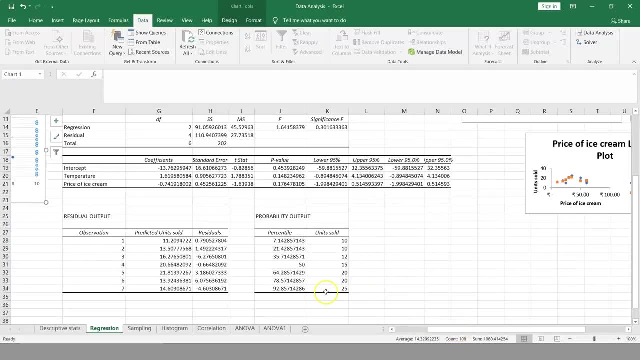 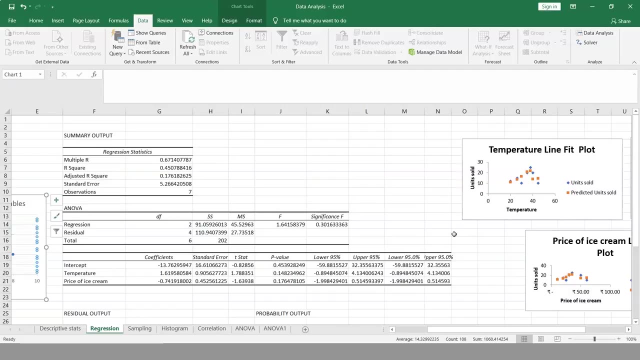 details to this particular plot and you also have normal probability plot, which is basically getting your values from your probability output here. so this is how you can perform a simple regression analysis, and now what you can do is you can, as i said, you can basically be looking at your scatter. 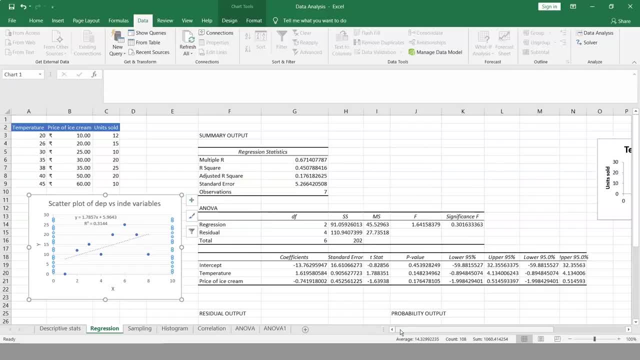 you can be looking at your y and x and your r square values, right, but remember what are the variables which you are selecting, and then you can compare these with, basically the values, what you see here. so remember, here i have chosen my both set of variables and you can choose one variable. 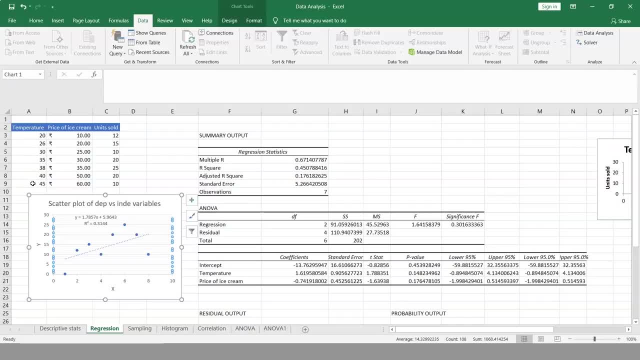 and then basically see what is its impact on the response or on the target. so it's pretty simple here. you can add more details to your scatter plot or the plots, what we have created, or some people prefer to do it using formulas. so basically we have some statistical functions that can help you do linear regression analysis, such 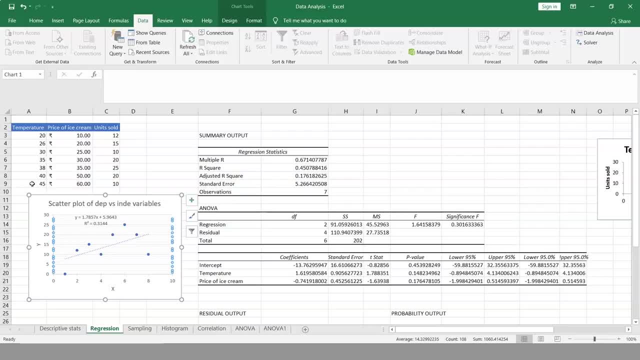 as you have linux, you have slope, you have intercept, you have correlation and so on. so basically, you can use these particular functions and what you will have to do is you will have to basically go in for a function if that's what you would want to do, and then you can search for functions. 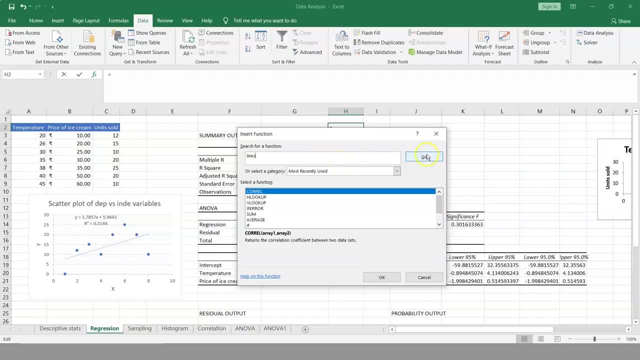 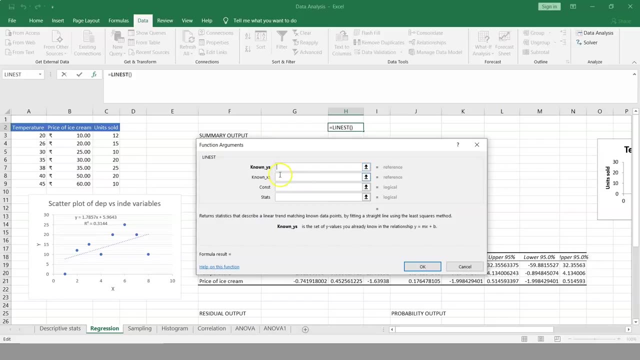 and say, for example, i'll just say linest and say go, and here i have my function. so if i would want to really use this one, i can do that. what i will have to do is then select the variable. so if you just say, oh, okay, and that basically says your known, wise, known x, your constants, your stats, and basically you can.